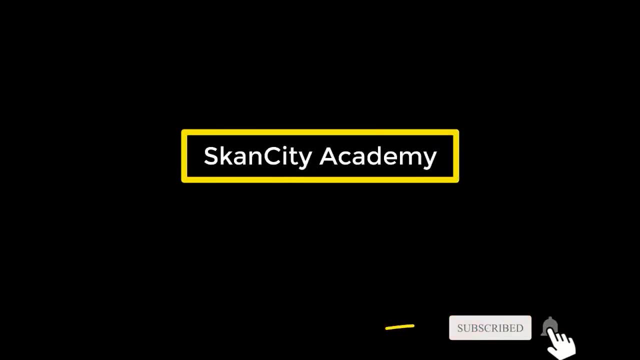 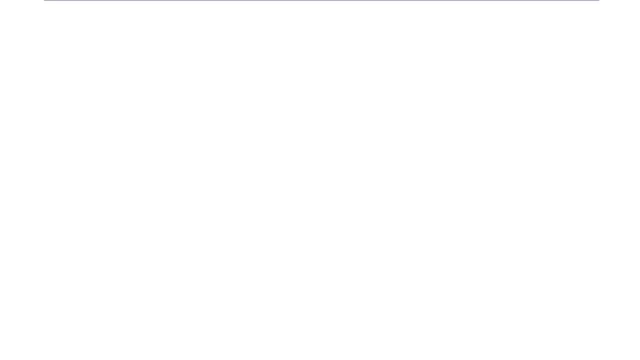 So in this video we are going to learn how to convert a complex number in the rectangular or cartesian form into the polar form. So, given a complex number, say z equals x plus j, y, Now let's call this equation 1.. And this is the rectangular or the cartesian representation. 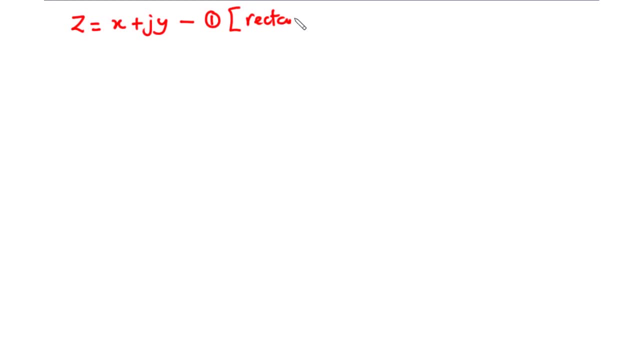 of the complex number, So rectangular, or the cartesian representation of the complex number. Now, at this point, we are going to represent this complex number on a graph, And this is made possible by the use of what we call the Argand diagram. This diagram helps us to represent a complex 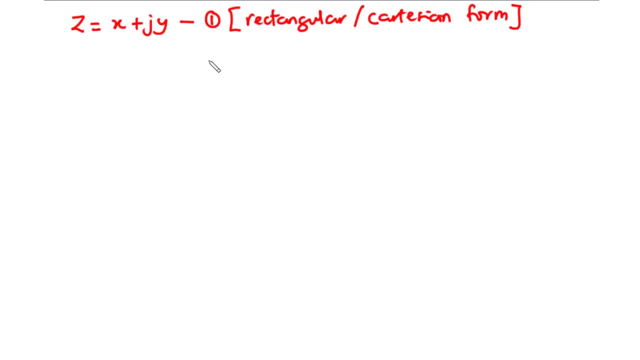 number in the complex number. So, assuming that this is the Argand diagram, we have the real axis and the imaginary axis, We have o to be the origin and we have the complex number, z, which is equal to x plus j, y, represented on the graph. 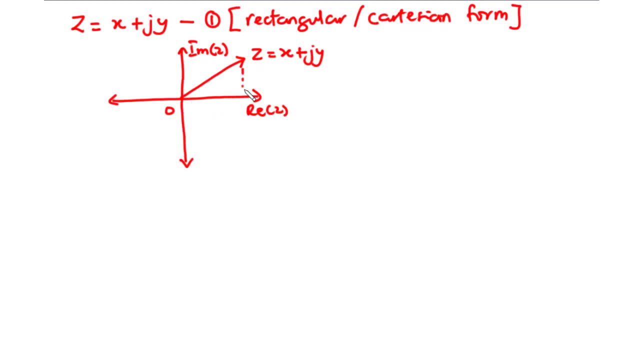 And the imaginary axis, we have y, and on the real axis we have x. We have r to be the hypotenuse and the angle theta formed between r and x. Now let's focus on this triangle. So from trigonometry we know that sine theta is equal to opposite over hypotenuse. 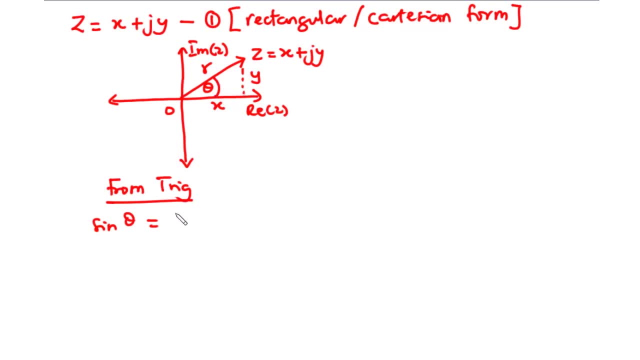 So opposite to the angle theta, we have y, So that is y over the hypotenuse is r, So we can say that y is equal to r sine theta. We have cos theta also to be adjacent over hypotenuse, So that is x over r. In that case we have x to be equal to r cos theta. 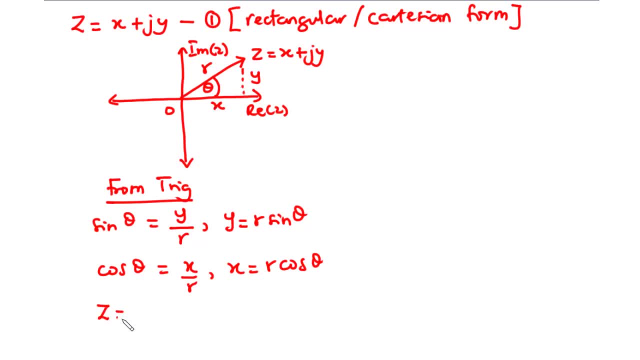 Now from equation 1.. We know that z is equal to x plus j, y. Now we are going to substitute the values of x and then y in here, So this becomes r cos theta plus j r sine theta. At this point r is common to both terms. 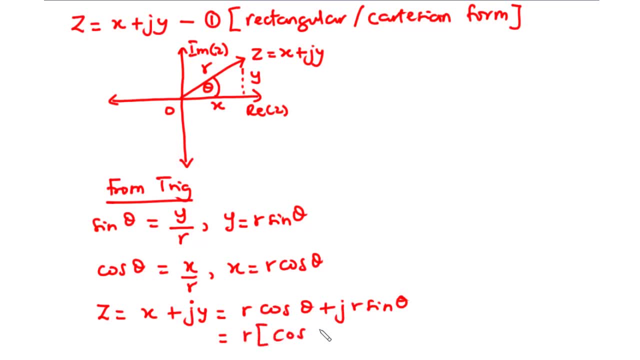 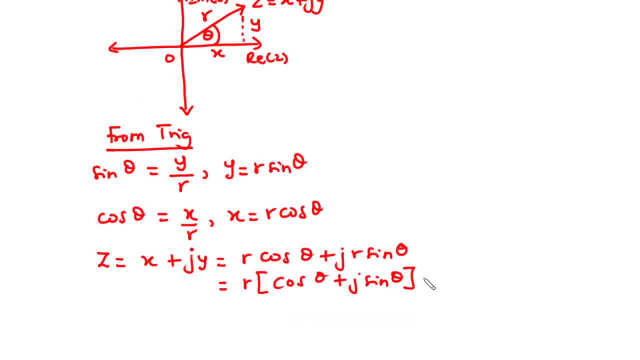 So we can factor out r, So that inside of the bracket we have cos theta Plus j sine theta. Now this is called the polar representation of the complex number And this can be reduced as r polar theta. So basically this is the shorthand form of the polar representation of a complex number. 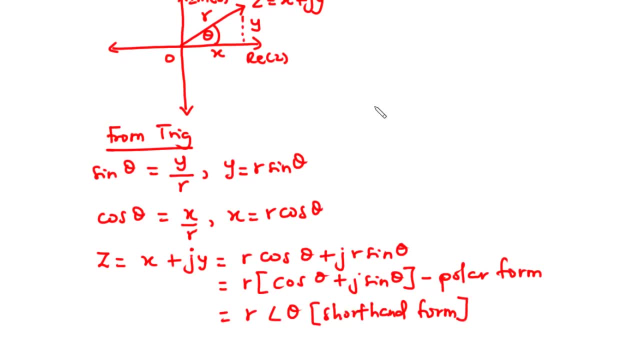 Where r is referred to as The modulus or the magnitude of z and thus written as mod z, or the absolute value of z. Also, theta is given by tan, inverse of the absolute value of the y component divided by the x component, And this angle theta. 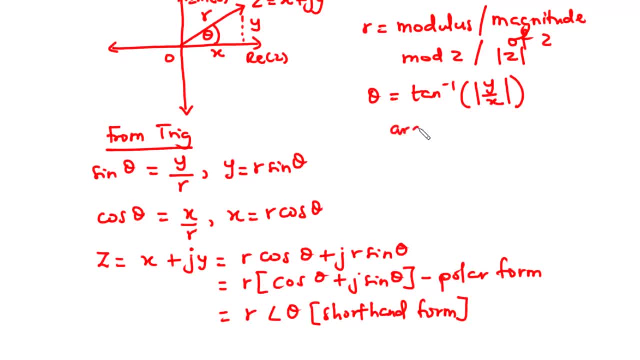 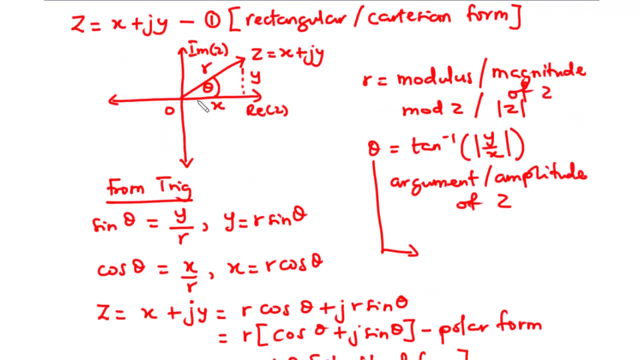 Is referred to as The argument Or the amplitude Of z. Now this theta is the angle z makes with the positive x axis. So theta is the angle z makes with the positive x axis, The positive X Axis. Notice that. 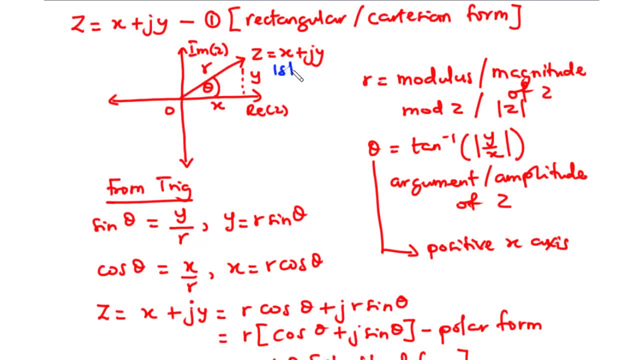 If z occurs In the first quadrant, Then we are going to use this approach To find the value of theta. However, if it appears In the second quadrant, The third quadrant Or the fourth quadrant, Then you need to perform further calculations. 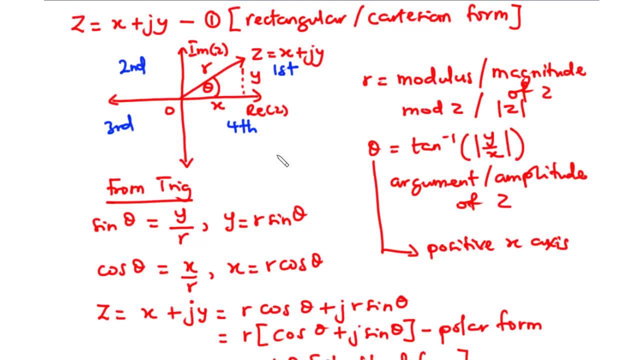 In order to arrive at the final value of theta. So, even before we take some examples, Notice that the value of x Is the value of r Can be found by using this formula: That is the square root of the x component square. 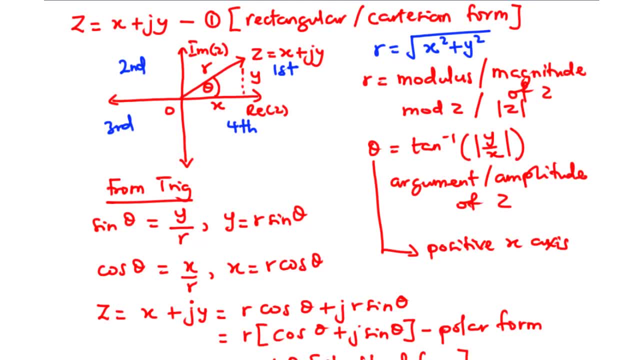 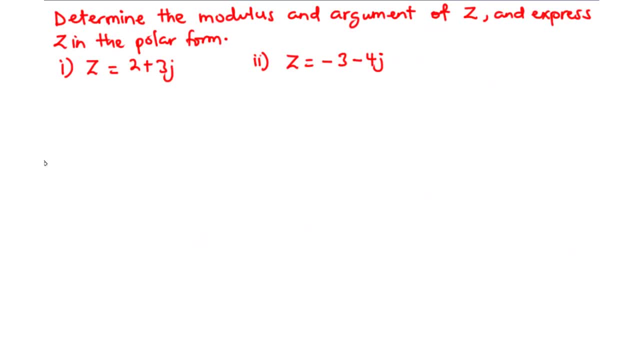 Plus the y component square, Determine the modulus and argument of z And express z in the polar form. So for i, We have z to be Two plus Three j. Now this is the rectangular representation Of the complex number. We need to convert this. 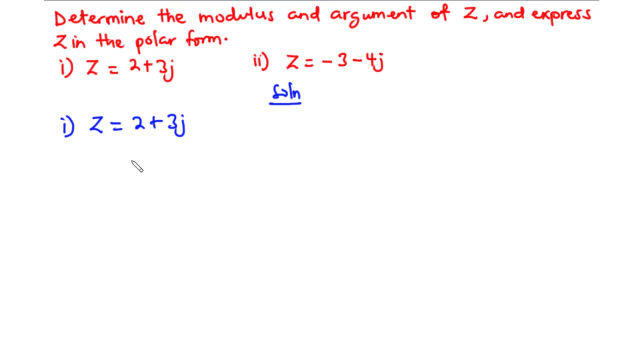 To the polar form. So in order to do that, First of all We need to draw the Argand diagram, We need to represent This complex number In the Argand diagram. So we draw our diagram, We have the real axis. 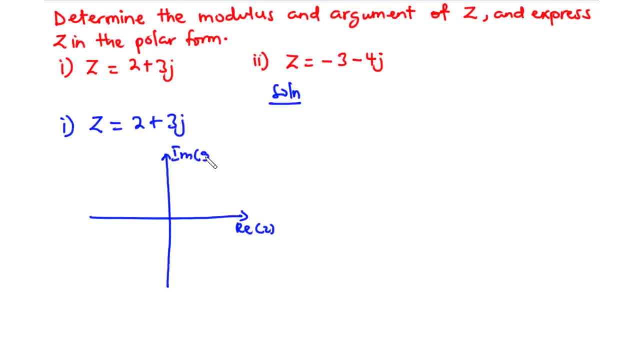 We have the imaginary Axis. On the real axis We have the x component, To be two, And on the imaginary axis We have three. So we have z, equals Two plus Three, j. This is the angle, theta, And then we have r. 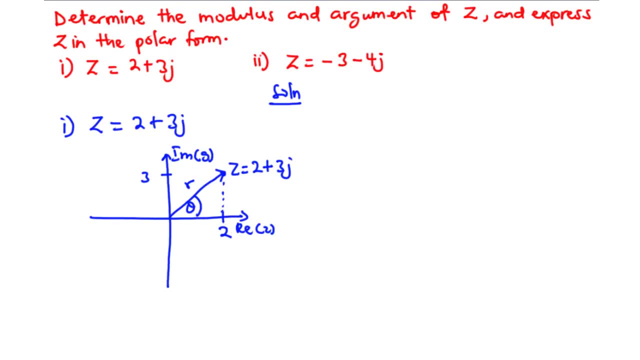 That is the modulus, And at this point You realize that The complex number Is formed in the first quadrant. But the complex number Appears in the first quadrant. Now let's move on To find the value of r And theta. 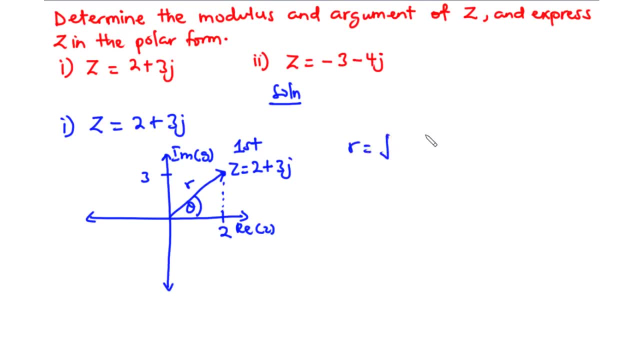 So we know that R is equal to The square root of X square Plus y square. We have x to be two, So that is two square Plus We have y to be three, So three square. So we have the square root of. 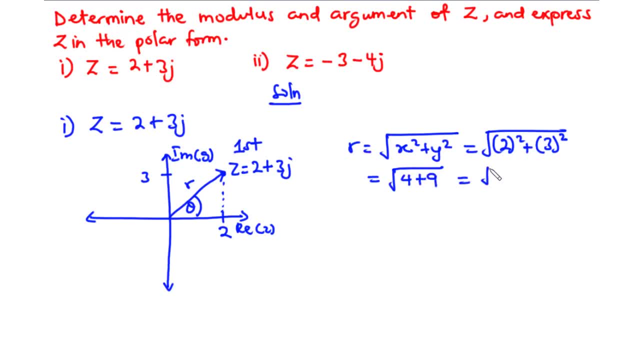 Four Plus nine, And that is equal to The square root of thirteen. So we have r to be The square root of thirteen units. Now let's find the value of theta. So theta is giving us Tan inverse Of the absolute value of y. 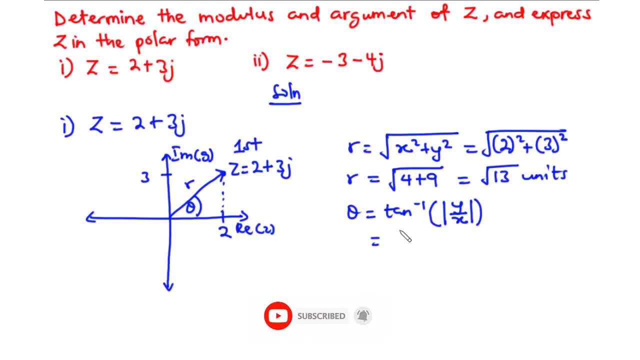 Divided by x, So this becomes Tan inverse of Three, And then x to be two, So tan inverse of Three over two Gives Fifty six Point Three one. So this is the value Of the argument. 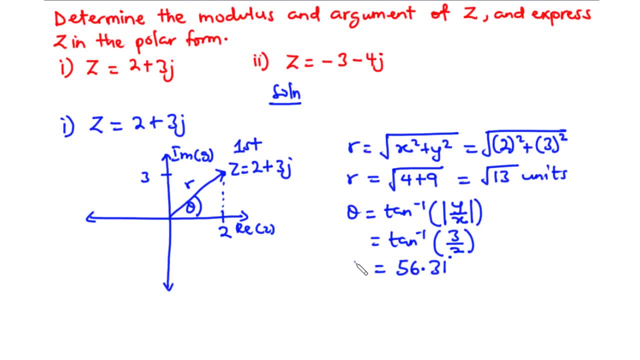 So now let's represent Z in the polar form. So we have Z equals R into bracket Cos theta Plus J Sin theta. So this becomes R Into bracket Cos theta Plus J Sin theta. 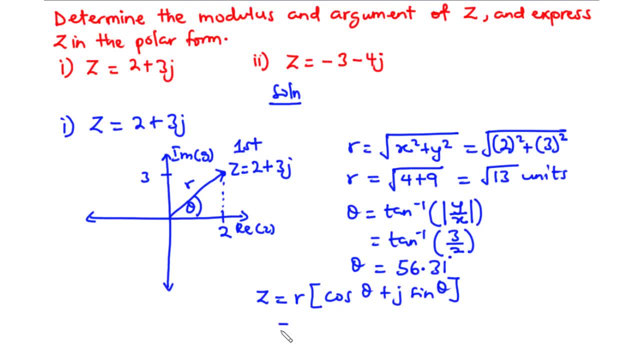 So this becomes R Into bracket, Cos theta Plus The square root of thirteen Times In a bracket We have Cos Fifty six Point Three, one Degrees Plus J Sin Fifty six Point. 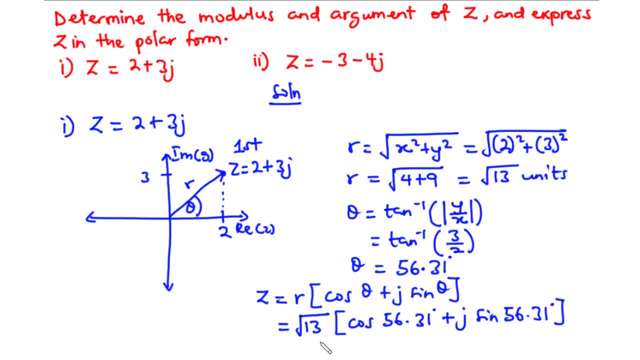 Three one Degrees, The square root of thirteen Polar Fifty six Point Three one Degrees. So this is The polar form Of Thirteen Degrees. So this is The polar representation Of The complex number. 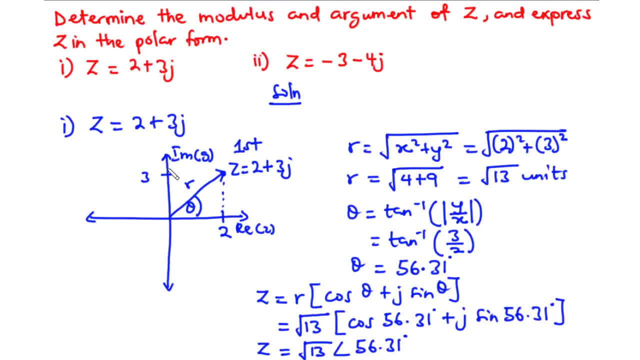 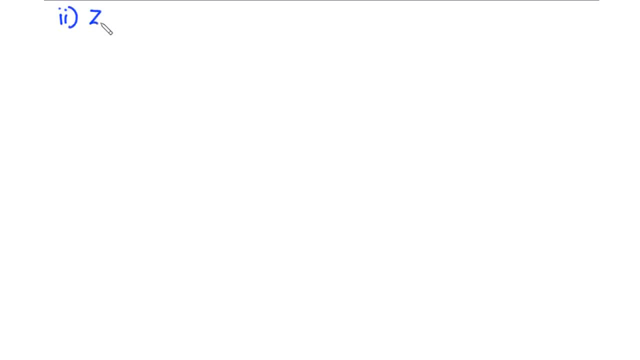 Two Plus Three J. Now let's move on to I I. So For I I, We are going to represent The complex number That is Negative Three Minus Four J. 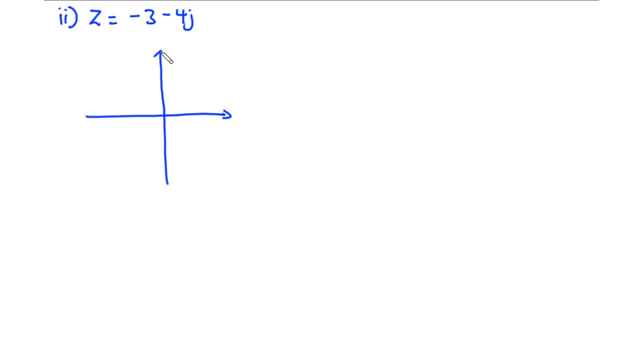 In the polar form. So we have This to be Our Argand Diagram. This We have The Real Axis. We have Our X Component To Be Negative Three. So This: 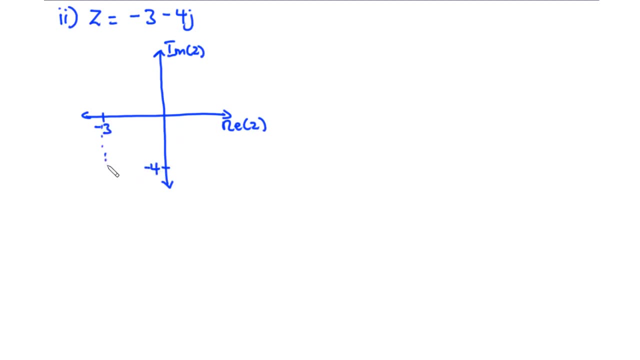 Is Negative Three. Y Component Negative Four. So This Is Negative Four. So This Is Negative Three Minus Four J, And This Happens To Be. 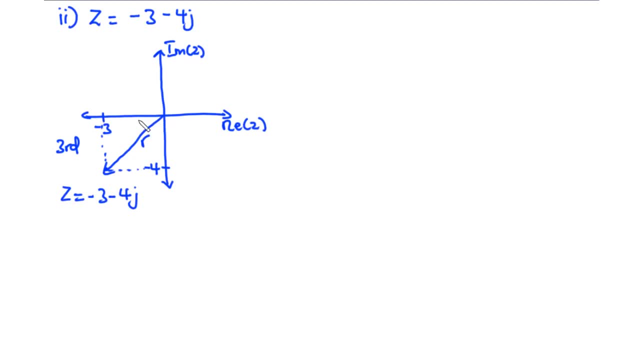 Formed In The Third Quadrant. We Have This To Be Our And Let The Angle Between Our And Angle Theta. So From This Point To 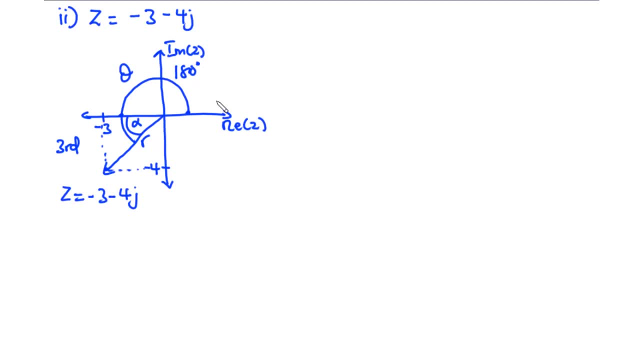 This Point Is 180.. Degrees, And Notice That We Always Move In The Anticlockwise Direction To Meet Our. So Now Let's Find So. 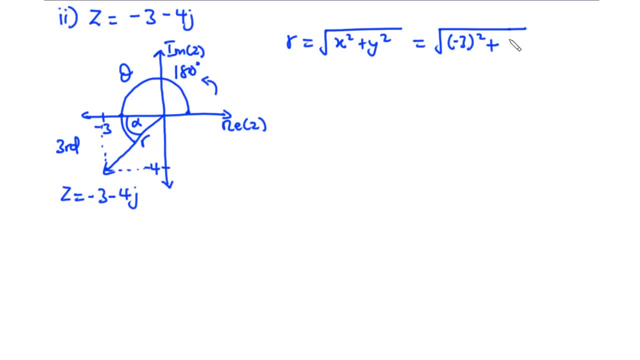 Negative Three Square Plus Y Is Negative Four, So Negative Four Square. This Is Equal To The Square Root Of Negative Three. Square Is Nine Negative: 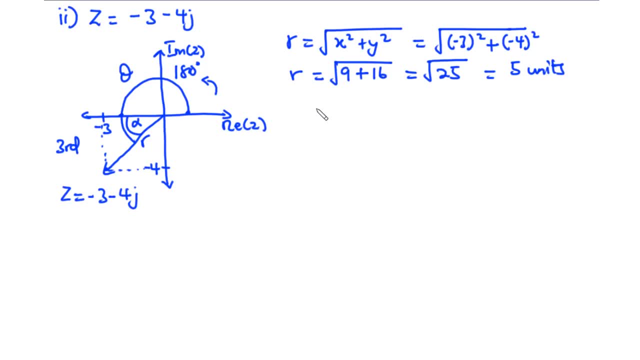 Four Square Is Negative, So Alpha Is Given By Tan Inverse Of The Absolute Value Of Y Divided By The Absolute Value Of X. This 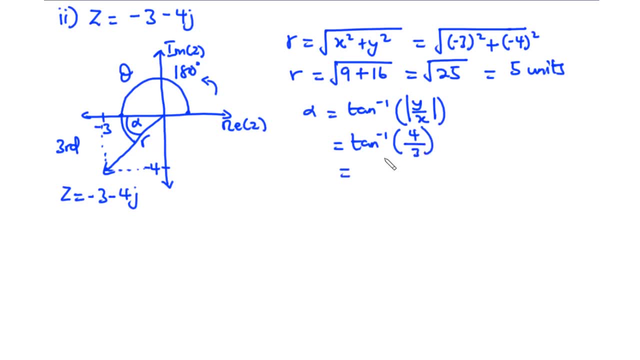 Is Equal To Tan Inverse. We Have The Angle, So This Is The Value Of Alpha, This Angle. Now, In Order To Find The Value, 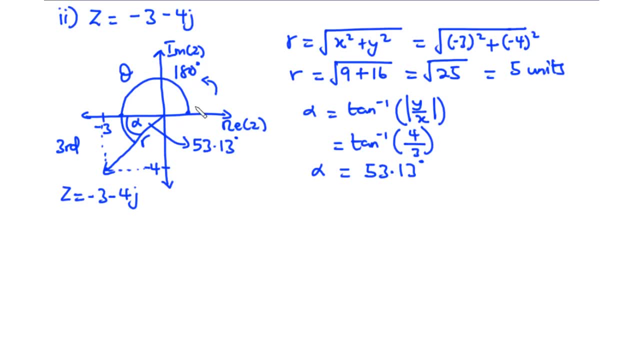 Of Theta. We Are Going To Add 180.. Degrees To 53.13.. That Is The Angle Theta. So Theta Is Equal To 180. Degrees. 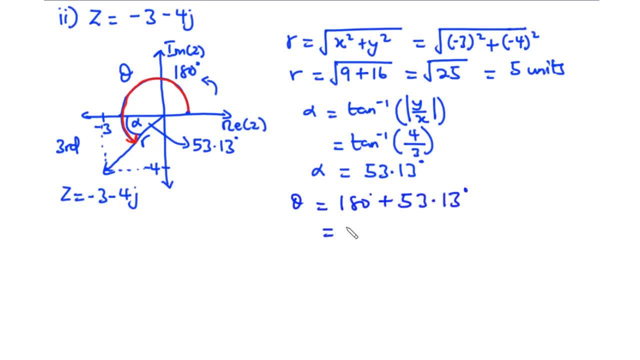 Plus 53.13. Degrees, And That Is Equal To 233. 13. Degrees. So This Is The Value Of Theta To Be 5.. Into Bracket. 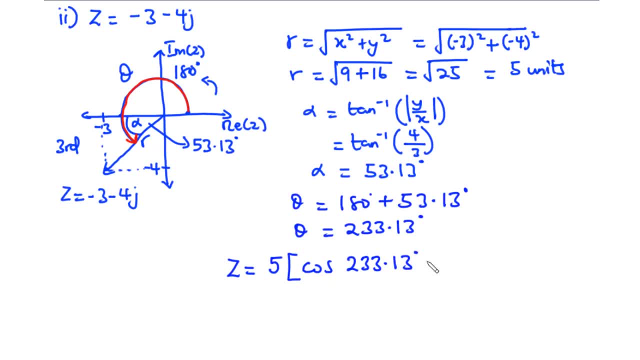 Cos 233. 13. Degrees Plus J Sign 233. 13. Degrees, Which Can Simply Be Expressed As: 5. Polar 233. 13. Degrees. So.